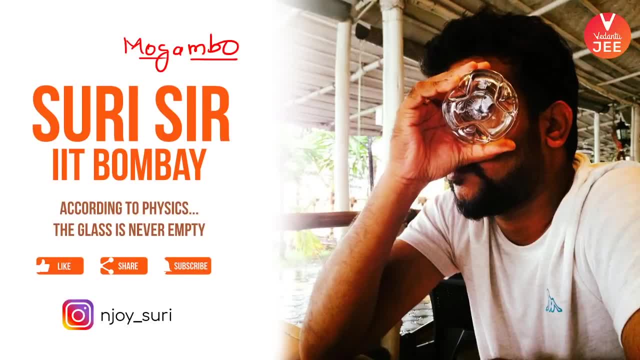 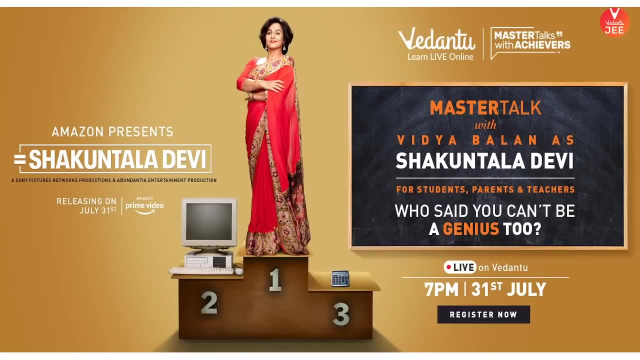 Wizard, Shakuntala Devi, in a movie by the same title, which is coming very soon on one of the OTT platforms, Yes, guys. so, without wasting any further time, let me first tell you that secret is getting unveiled. Yes, guys, in the next MasterTalk, after having Deepika Padukone. 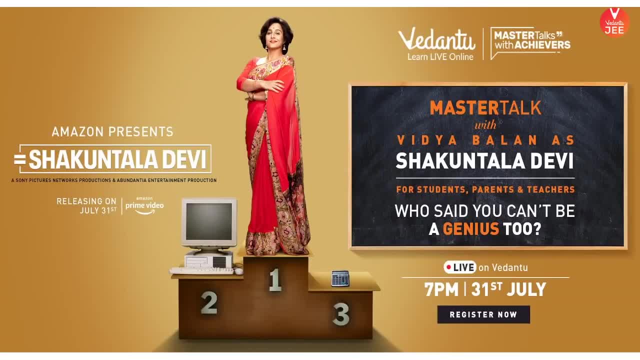 now we are bringing Srimati Vidya Balan, as she is playing Shakuntala Devi. So, guys, let's begin Chakuntala Devi. okay, so she is going to come live on 31st of July- yes, this next Friday at 7 pm. 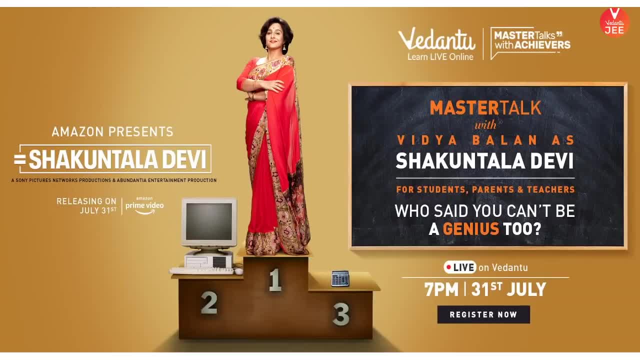 on your very own Vedantu platform as the master talk with achievers. so, guys, if, like me, you are a person who's fascinated by the math magic, then definitely you must have heard about Chakuntala Devi and certainly you would want to interact with the person who is playing the role of that. 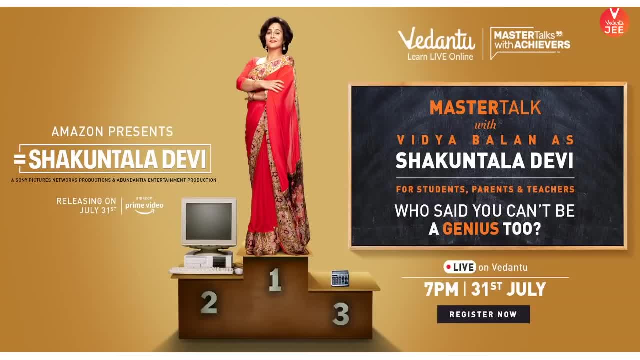 iconic person, right, guys? so put an alarm, put a reminder on your cell phone, set it at 7 o'clock, in fact, 15 minutes before that, for 31st of July, and I am going to watch it. I am sure you are also going to, definitely, okay, guys. so stay tuned to this channel and if you want more updates, 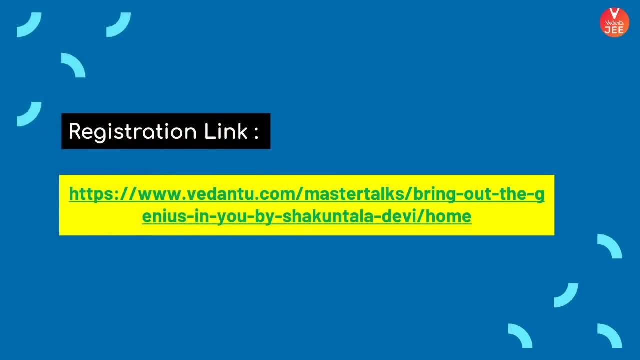 definitely. I would want you to subscribe to my channel and I will see you in the next video. subscribe to the channel as well. and, yes, this is the registration link. on this registration link, if you will click, you will be able to register for the session which is going to happen on 31st. 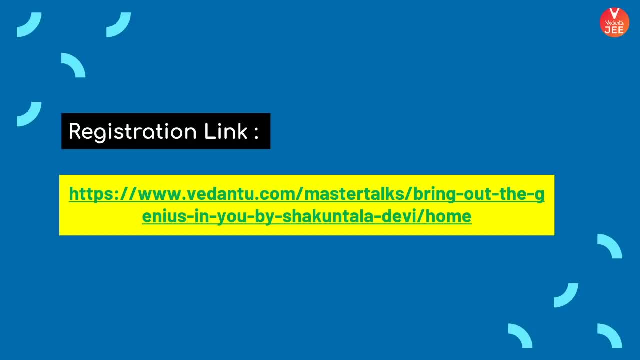 of July at 7 o'clock. yes, definitely, you need to register on this, guys. so where will you find this link? this will be available in the description box of this video, also in the comment section. okay, guys, so you will find that you guys are tech savvy. you will be able to find out the link which: 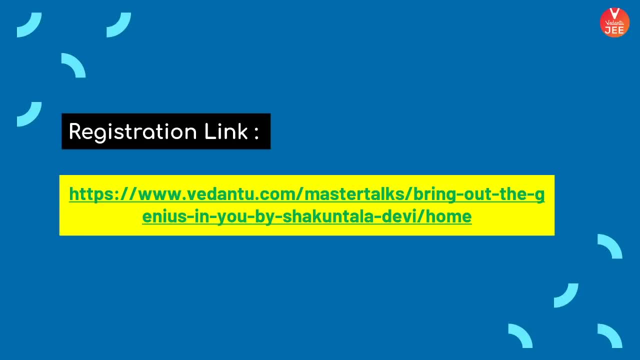 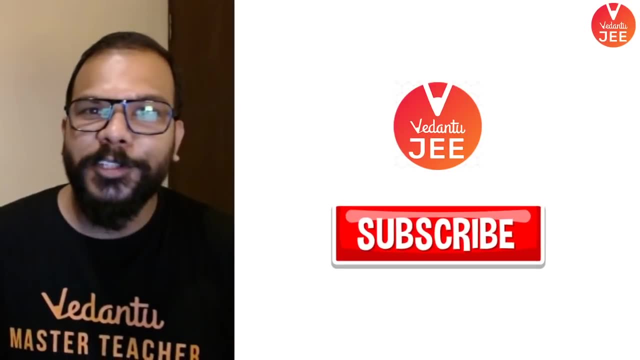 is available in the description box of this video. okay, guys, cool, and if you want to stay tuned to all these updates, as I said, do subscribe to the channel right now and press the bell icon so that, whenever all these awesome things are happening on this channel, you get to. 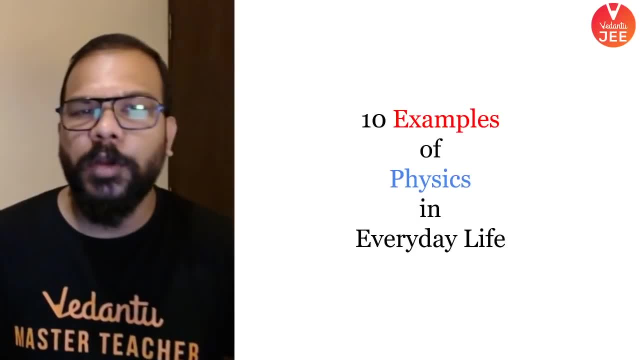 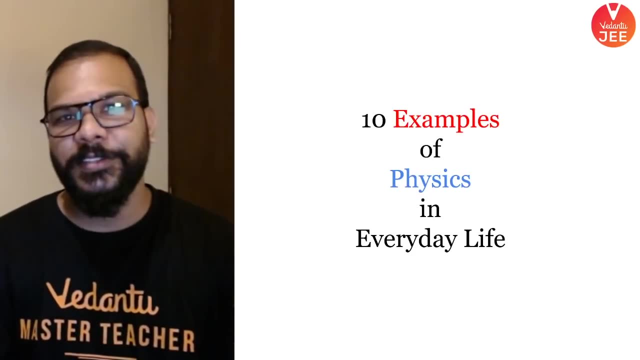 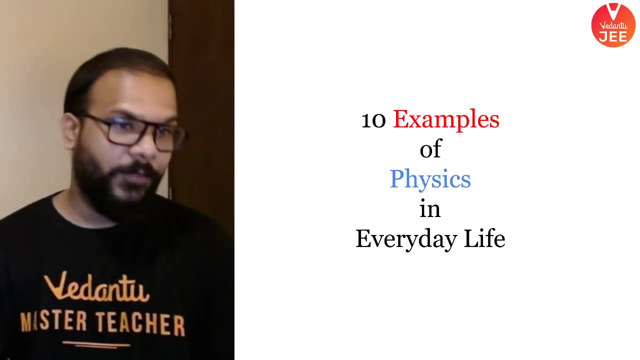 know that, okay, cool. so let's go forward and speak about the 10 examples of physics in everyday life. aren't you excited? I am, so this will be one of the most fun sessions to do here, because it gives me an opportunity to make you look at things from a different angle, from something. 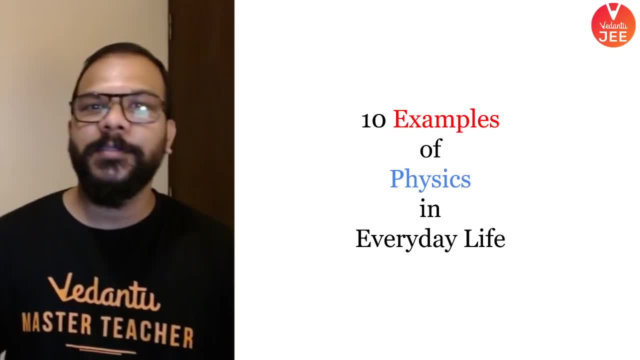 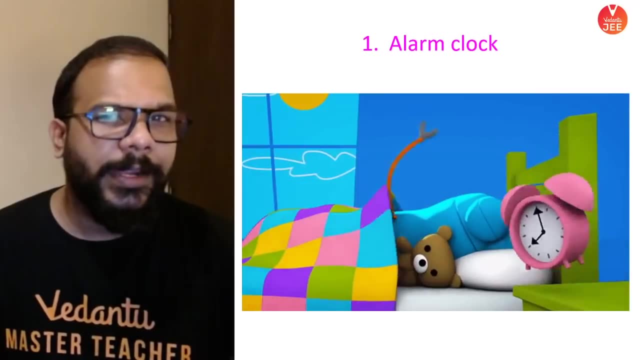 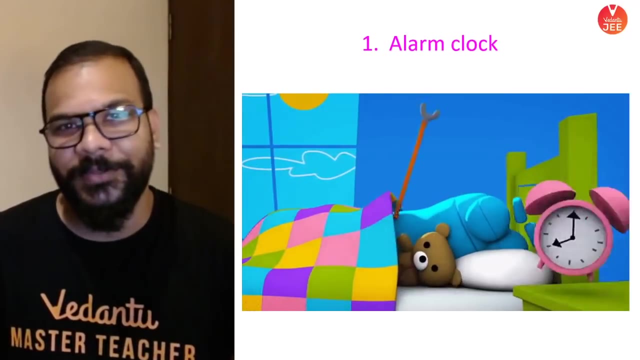 which we usually don't look at as a layman. so, guys, without wasting any further time, here comes the very first example, and that is an alarm clock. now, obviously, there are different, different ways of looking at an alarm clock, but just close your eyes and think about the morning, every morning, when that alarm clock goes off. what? 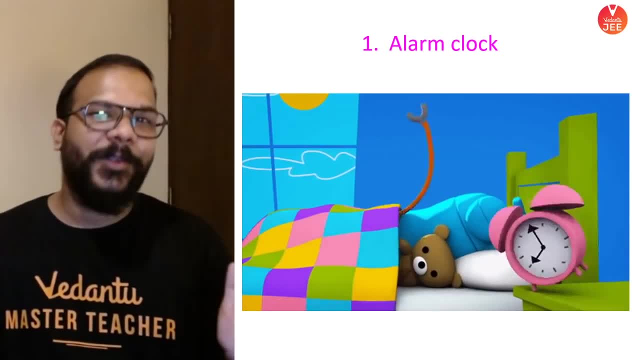 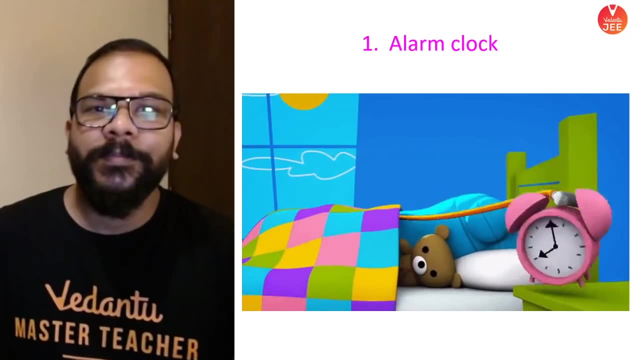 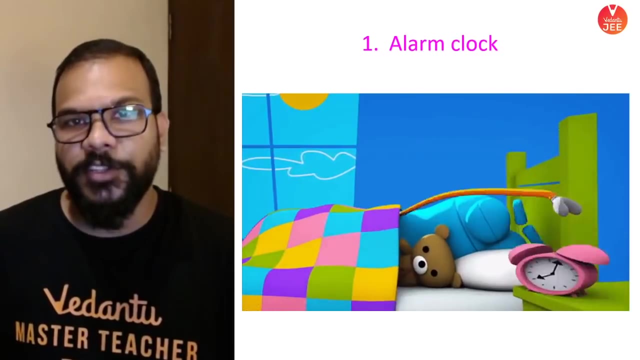 happens at that point of time. the alarm clock, the annoying sound of it, it wakes you up, right guys? so an alarm clock definitely is a mechanical machine, but the working principle, which is able to wake you up, is lying in the wave nature of sound. yes, sound is a mechanical wave, and alarm clock at. 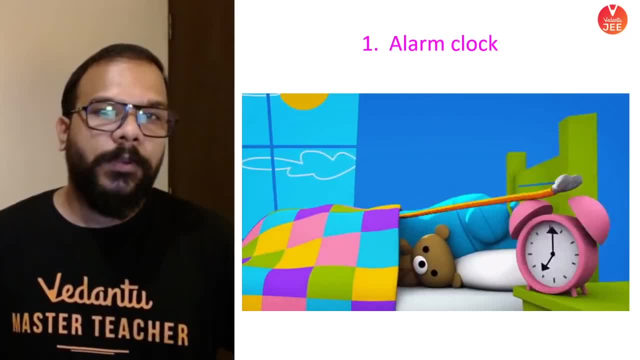 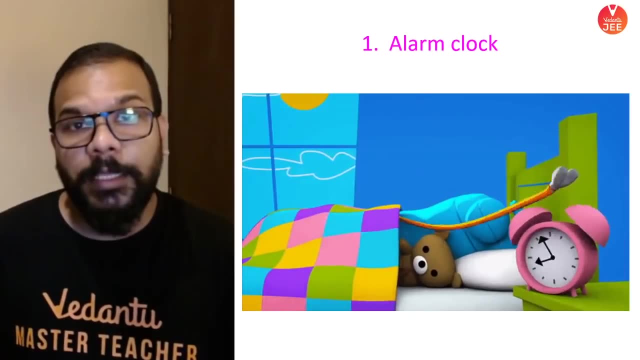 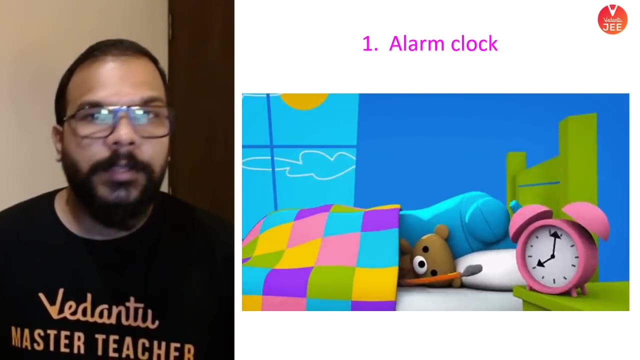 a mechanical level produces those sound waves of definitely a very, very, very high frequency, relatively a shrill voice, shrill sound which wakes you up. this is something that you learn in 11 standard in a chapter called as waves. that is where you get to know how sound waves as a mechanical 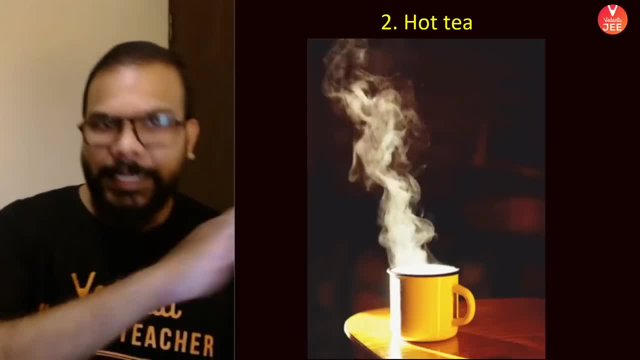 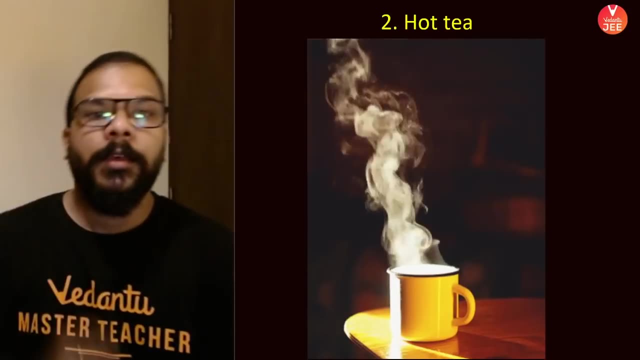 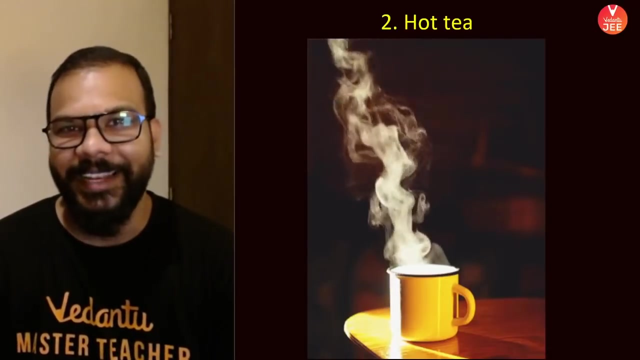 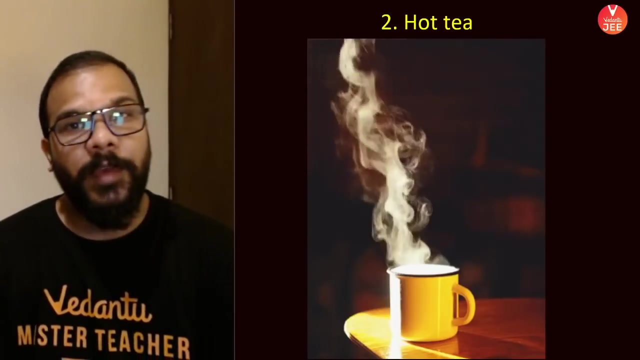 wave propagate through a medium okay. second example is how a hot cup of tea gets colder. so this is something which commonly you get to know in chemistry, but you study a lot about it in physics as well. yes, guys, the law is nothing but law of thermodynamics. what does it say? it says that if you have any hot object. 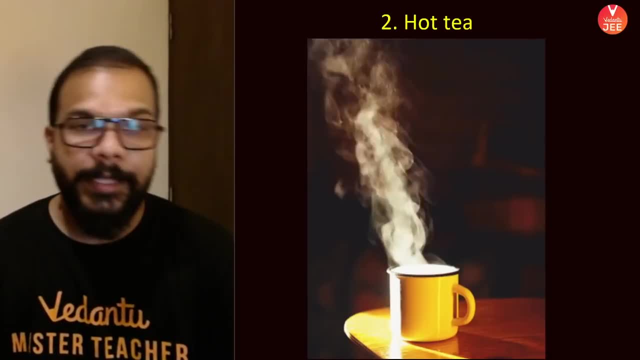 coming in contact physically with any cold object, then there will be transfer of energy from hot object to cold object, and that is how a hot cup of tea gets colder. so this is something which commonly you get to know in chemistry, but you study a lot about it in physics as well. yes, guys, the law of 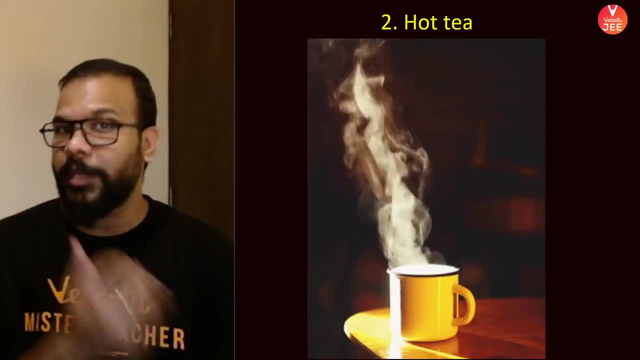 thermodynamics. what does it say? it says that if you have any hot object coming in contact physically with any cold object coming in contact physically with any cold object, in this process the temperature of the hot body will fall down. the temperature of the cold body will rise up till the time. 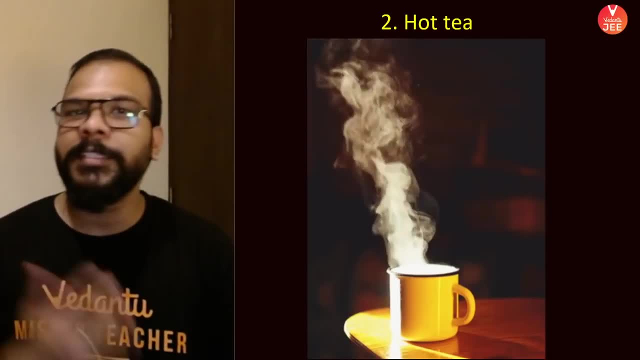 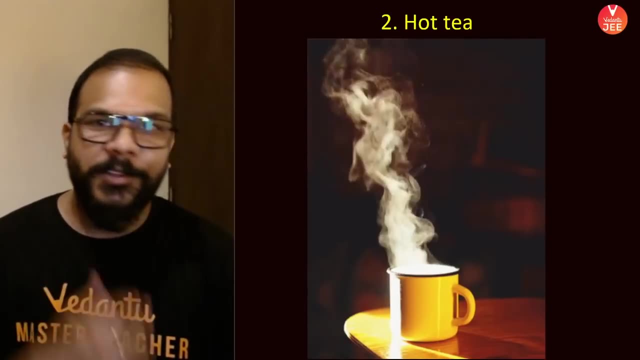 they both achieve the same temperature, which we call as the situation of thermal equilibrium. so that is why that hot cup of tea: if you are not consuming it, if it is placed on the table, it will get colder, only colder enough that it achieves the same temperature as the room temperature. okay, guys, 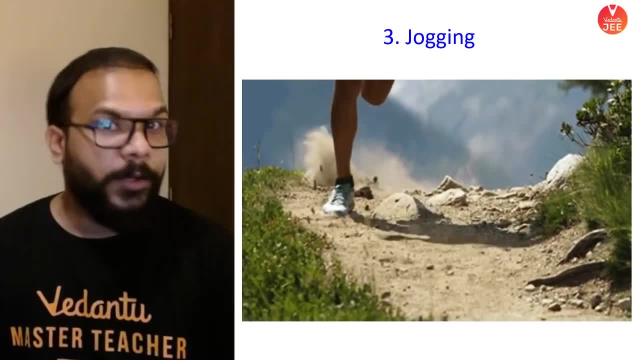 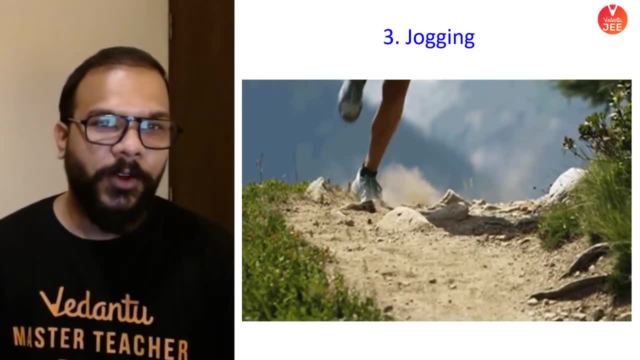 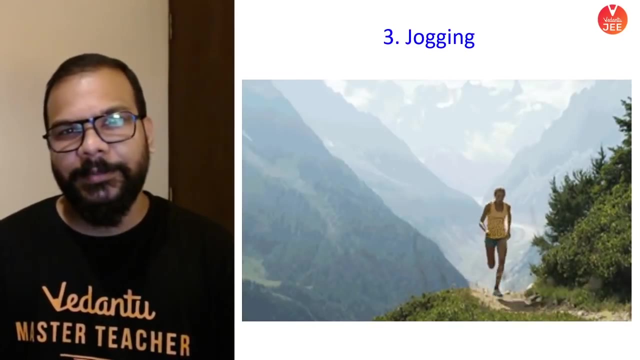 cool. next one: i don't know whether you do that or not. during this pandemic, definitely, most of us are not able to go out, even for a good jogging. but then when we look at the physics behind it, the basic reason of anything moving, as you know, lies in the 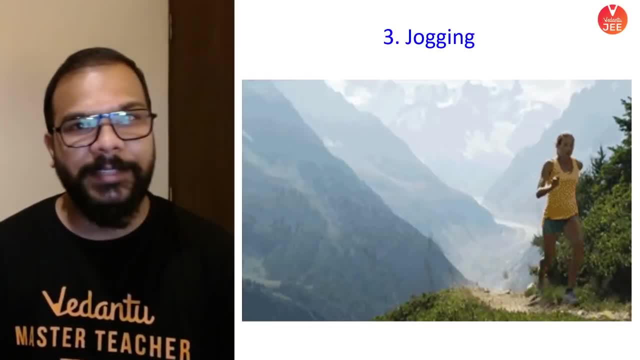 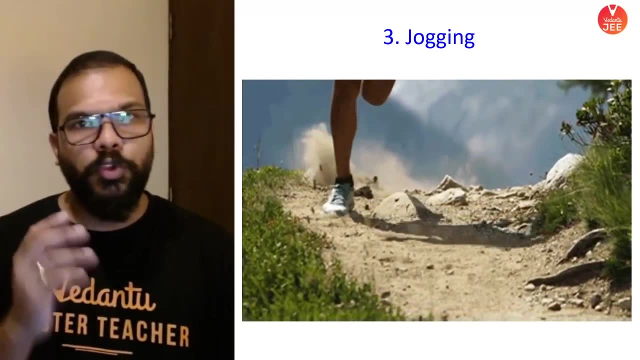 newton's laws of motion. so here also, the reason, fundamental reason why we are able to jog or walk is the newton's third law of motion. yes, guys, when you try to move, you push the ground from one of the legs. the other leg, as you can see, is always moving, and when you try to move, you push the ground. 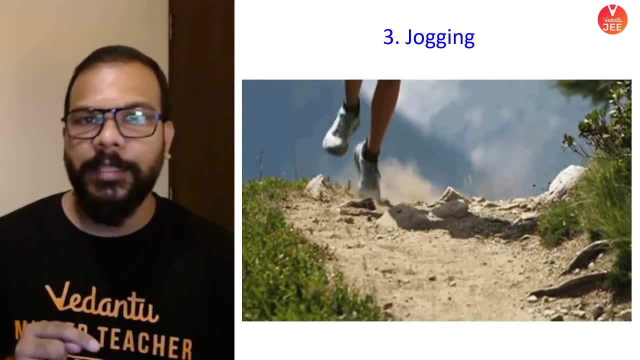 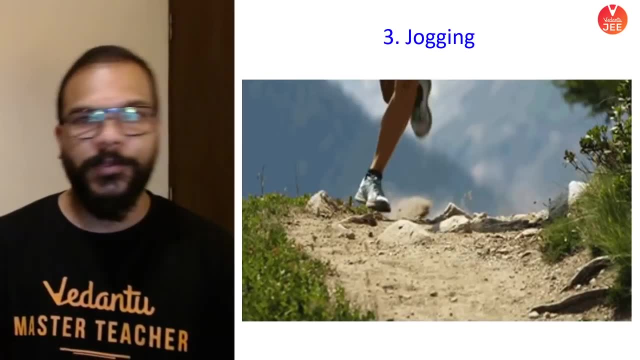 in air right. so the leg, which is in contact with the ground, tries to push the ground back. you apply an action force on the ground as a reaction. ground applies a reaction force on your body and hence you move forward. that's what you actually do whenever you walk or you jog. okay, 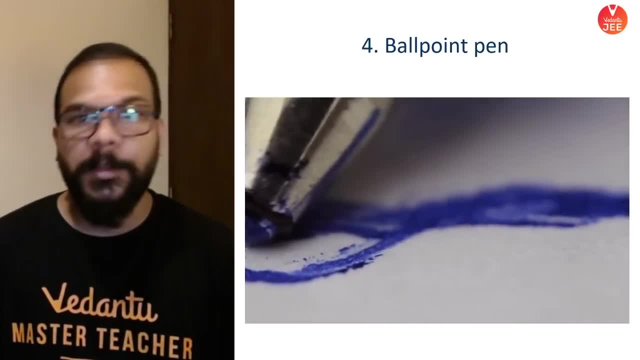 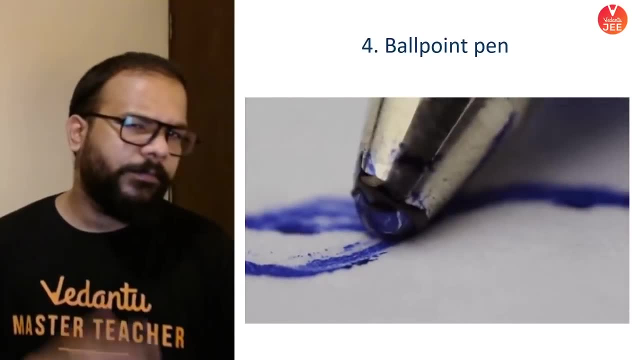 okay, now the third one is the working of a ball point pen. now, this is something which i'm sure most of us do not know about. so the fundamental reason- in fact i speak about a fundamental reason- of working of ball pen is the design of the ball. 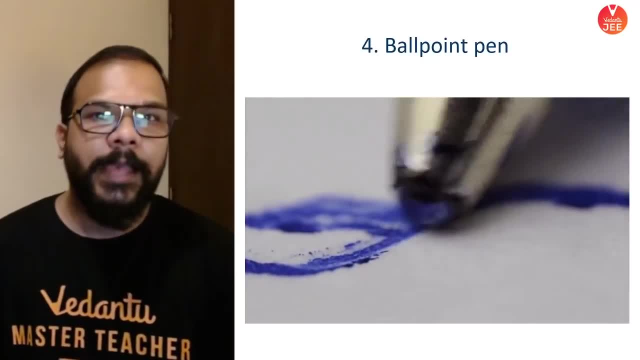 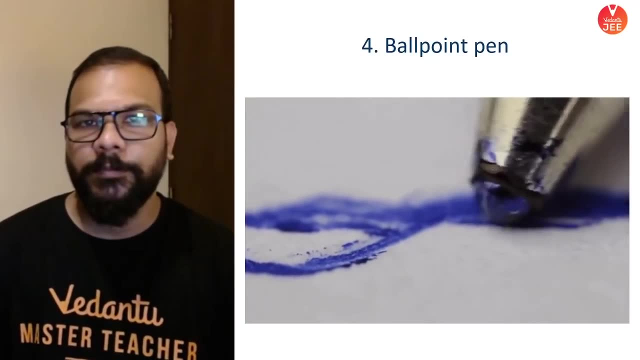 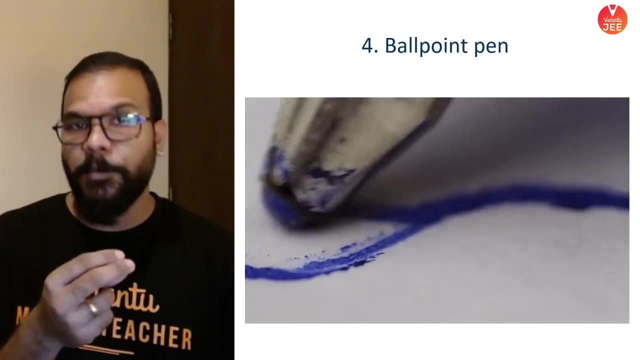 pen itself. so if you are able to see this animation right now properly, you see there is a spherical small point object which is at the tip of this pen and that is why it is called as a ball point pen. so this ball which is at the tip of the pen, or the refill whenever you try to write. 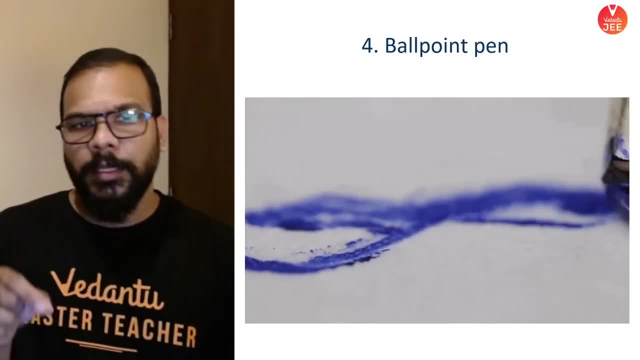 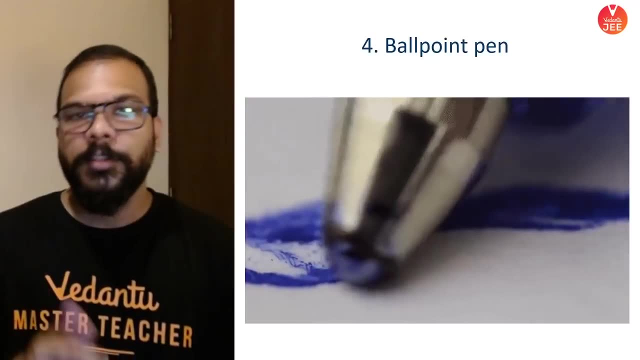 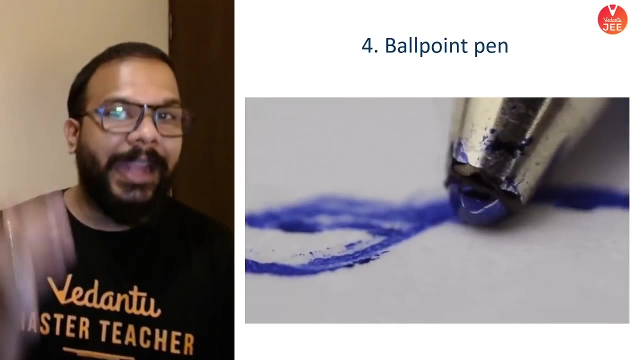 anything on the paper. you fundamentally are moving the pen on the paper by bringing it in contact and you are actually moving that pen and in this process you are making the ball roll. so when the ball rolls, there is certain gap which is there between the ball and the filling. because of the gravitational effect, the ink flows down. 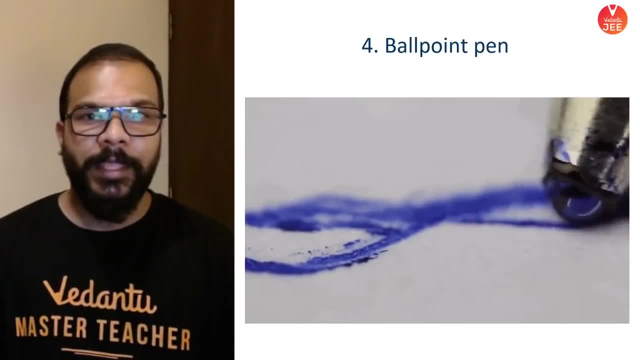 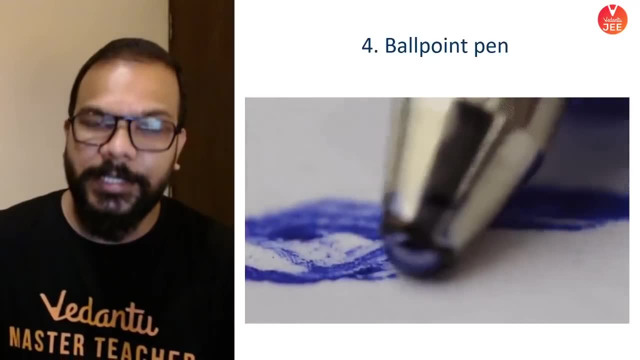 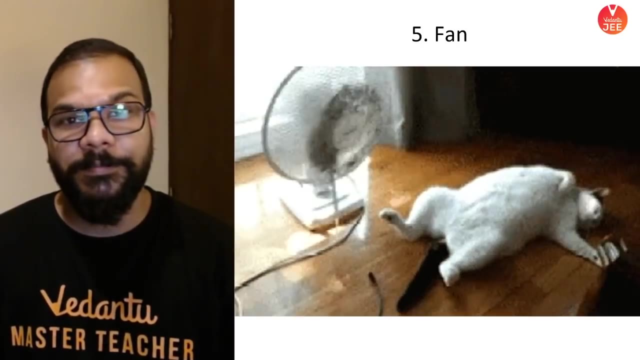 and that makes the writing possible. have you ever tried to write upside down? guys, take a paper like this and try to write. you will not be able to write. why? because it's the gravitational force which makes the fluid come down. okay, how about this? yes, one of the most needed thing during the 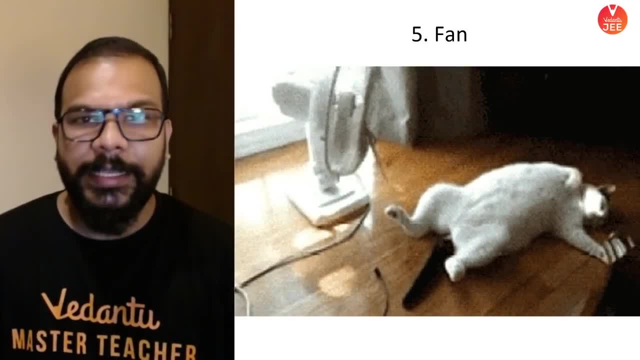 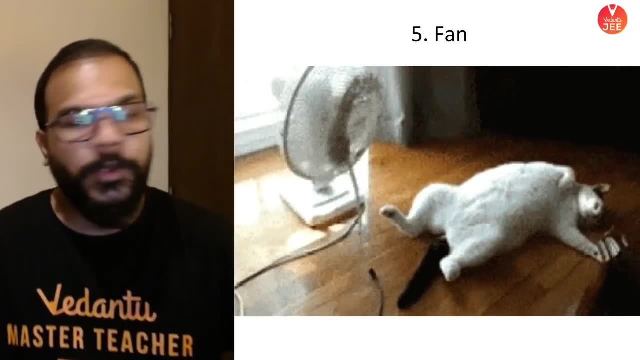 time of summers and, in general, for any other time than winter, is a fan, or in fact, if i have to speak, it's actually any machine which can rotate. so any machine which can rotate, including a fan or a mixer grinder or the dryer of a washing machine. 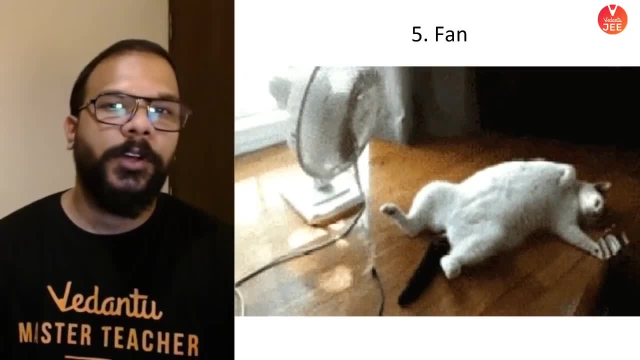 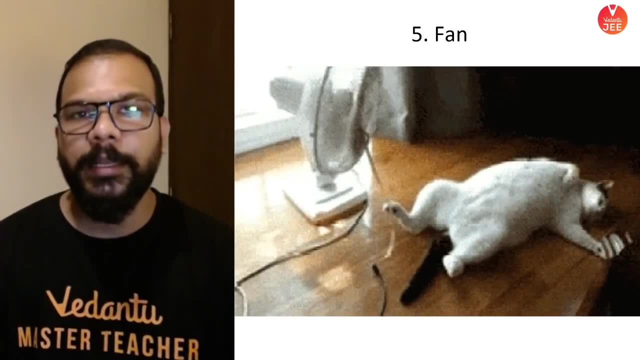 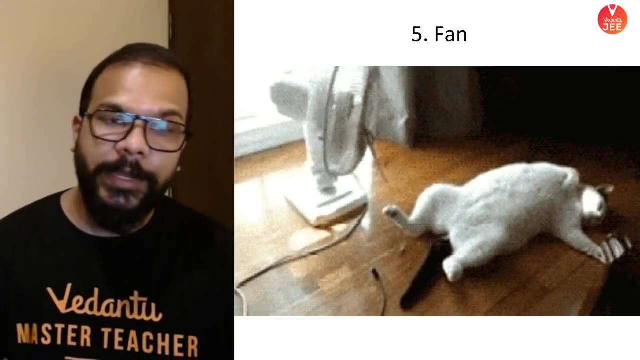 any machine which can rotate. it works on the principle of electromagnetic induction and in that also you will learn a concept in 12 standard where you will have a current carrying loop or a coil which if it is placed in an external magnetic field it starts to rotate. okay, so it's basically working on. 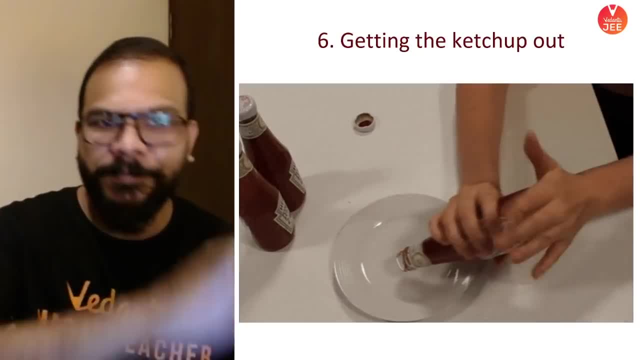 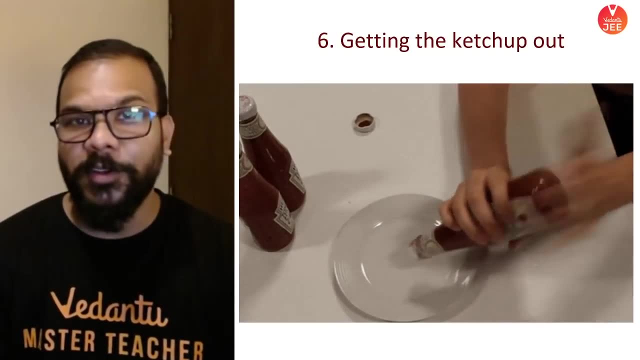 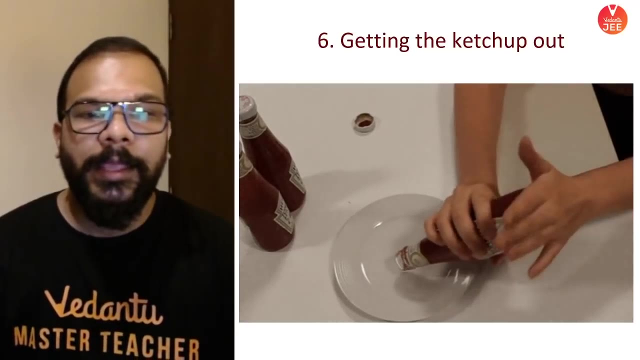 the principles of electromagnetic induction. next thing is: uh, yes, that ketchup bottle that you are trying to bring that ketchup out of the bottle. what you try to do, you, yes, you try to shake that bottle or you try to push it from the back of the bottle. in this process, can you think of what's happening? 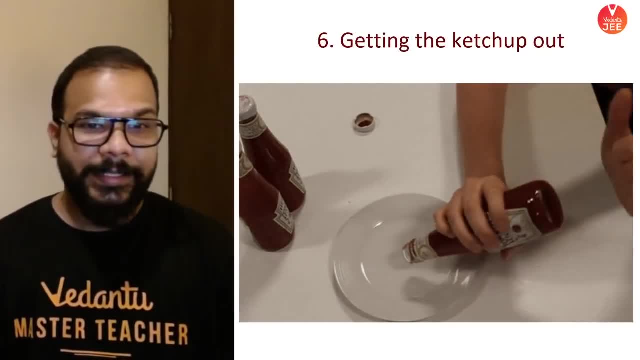 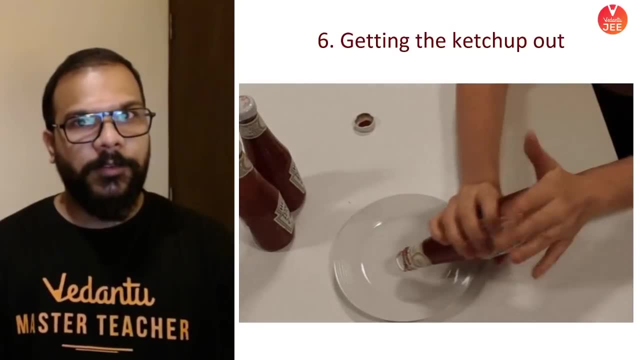 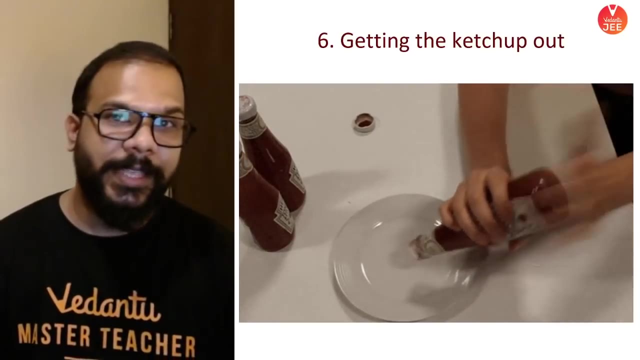 this is again newton at its best. this is the first law of motion, right in that we know that first law of motion is law of inertia. you are actually applying a force on the bottle, but you are not physically touching the ketchup inside. you are actually applying a force on the bottle, but you 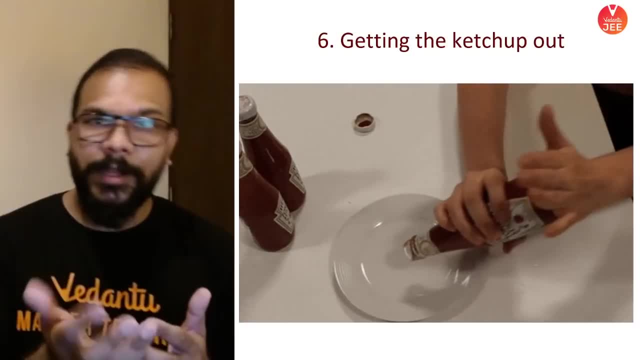 are not physically touching the ketchup inside. you are actually applying a force on the bottle. but you are actually applying a force on the bottle, but you so when you are pushing that bottle forward. so when you are pushing that bottle forward, it goes forward. then it tries to come back. 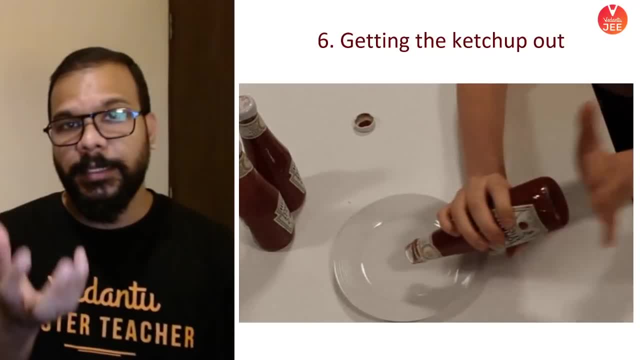 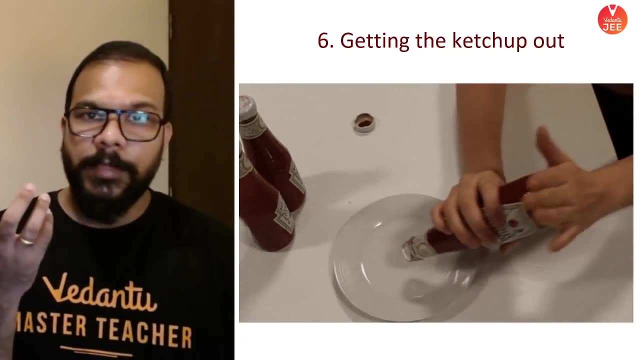 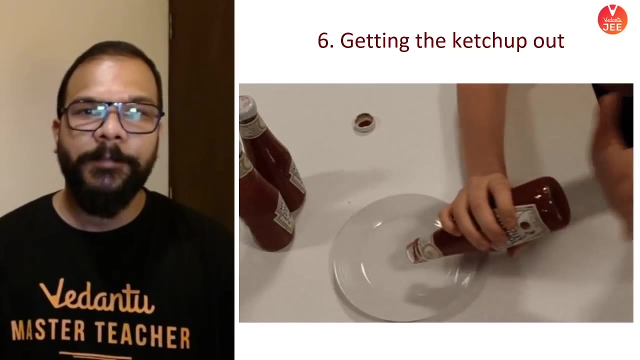 right in this process, when you are hitting it again and again, the liquid sauce which is inside. it is because of inertia, trying to maintain its position. when that position is vacated by the bottle moving forward and backward a bit, the liquid goes out because of, again, the property of. 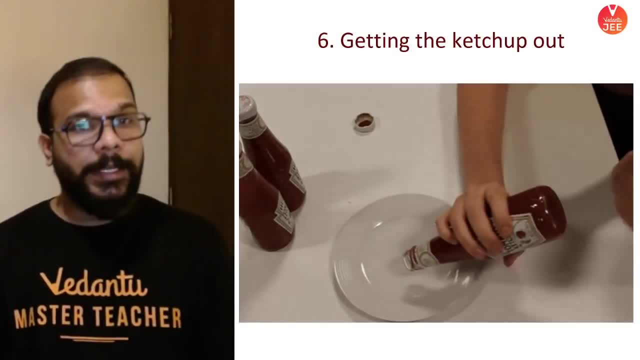 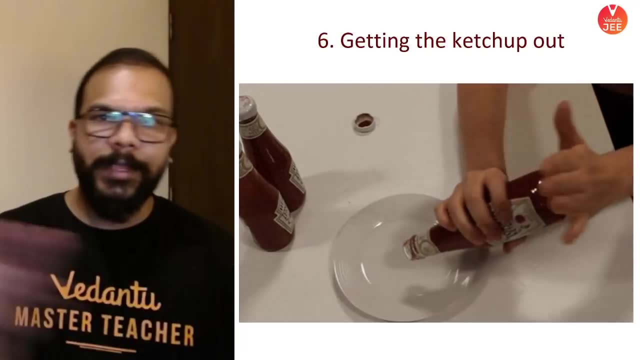 its inertia, and the first law of motion makes this possible. in fact, similar example is valid. valid when you try to clean a rug by beating it, so the dust particle wants to stay there, but the rug keeps on moving, so this makes the cleaning possible. this separates out the two objects. 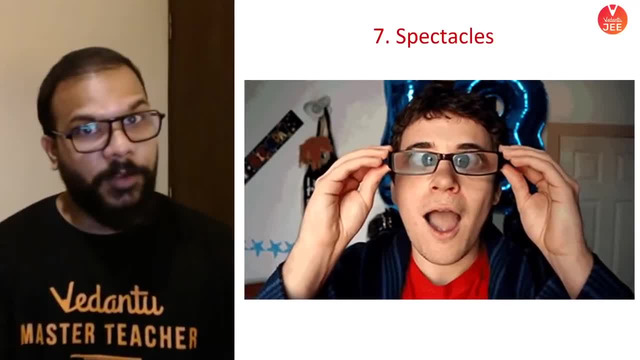 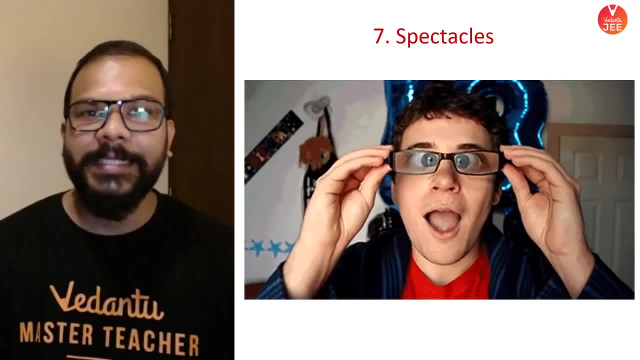 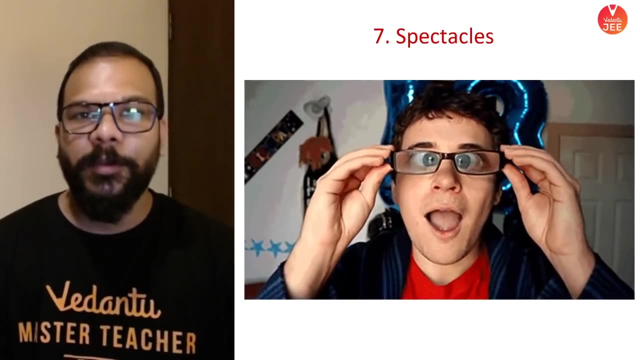 okay, moving on. yes, something from optics, your specs, how you are able to see, how am i able to see clearly right now is one of the magics of the unit of optics. this is i am sure you have heard about, you have known this also. it's the phenomena of refraction. 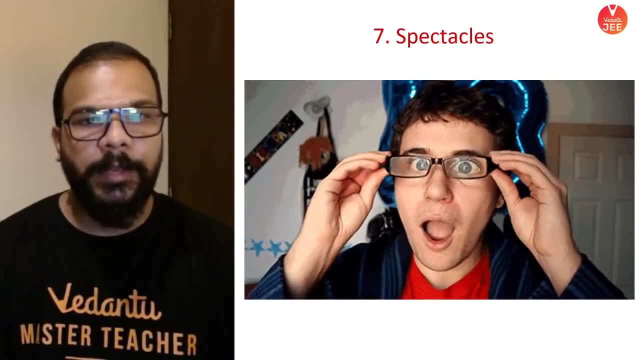 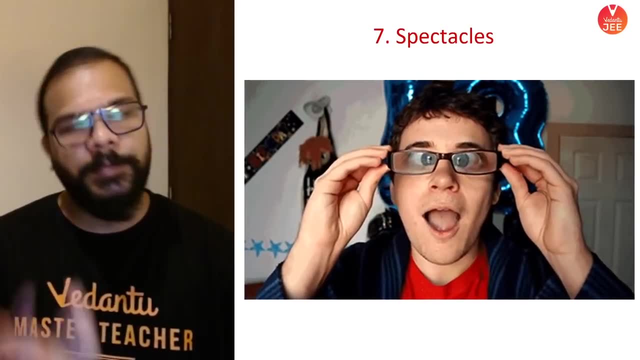 through spherical surfaces, because of which the light will bend and will create magnification effect, because of which things which were smaller will look bigger, or things which were not clearly visible will also start becoming visible to you. so it's optics at its best, and that to refraction. 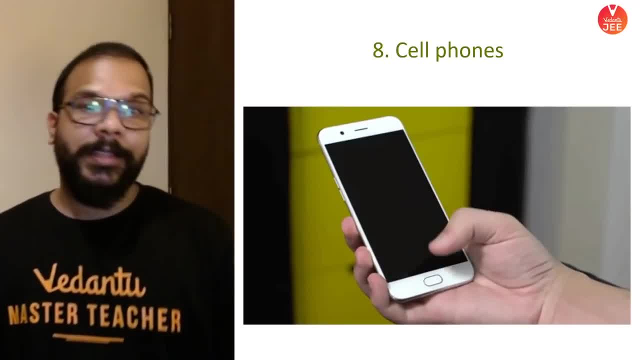 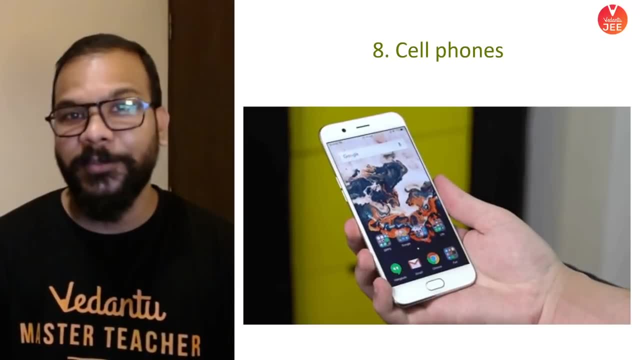 the basic reason behind it. how about the device which is keeping us connected, the device which is a must in the present generation? yes, your cell phones. a cell phone is, I would say, a magic of modern physics. that means Albert Einstein era, Any cell phone or any. 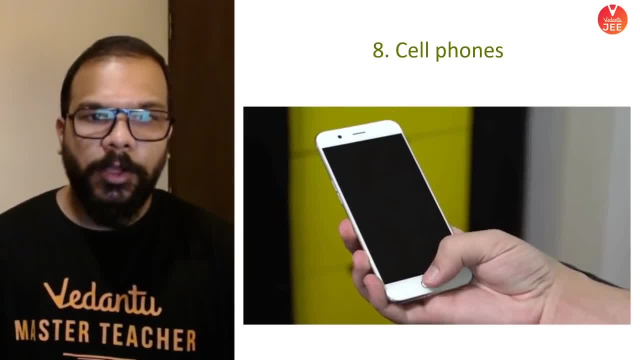 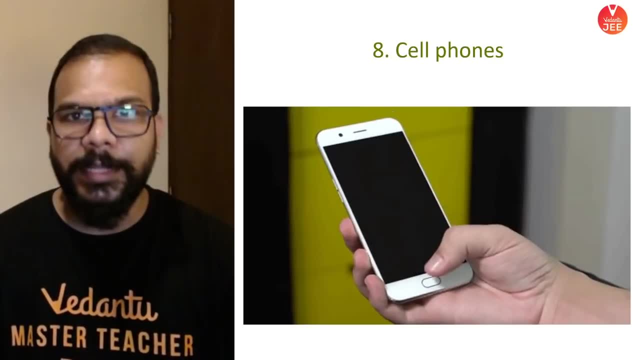 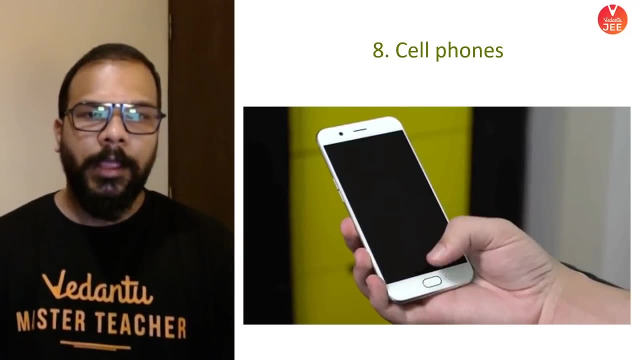 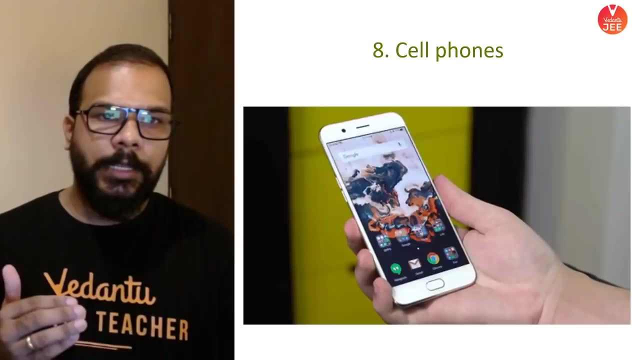 electronic device, for that matter, is working on the basis of the modern physics electronic structures or the electronic circuits that we deal with. In addition to that, your cell phone becomes that more helpful and it actually lets you connect with other people because, beyond the electronics, it actually works on the communication system where you have radio waves getting. 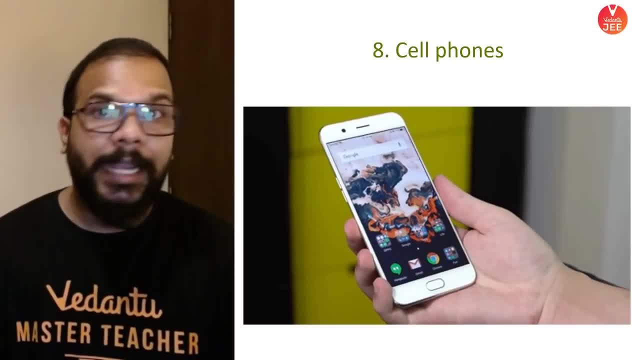 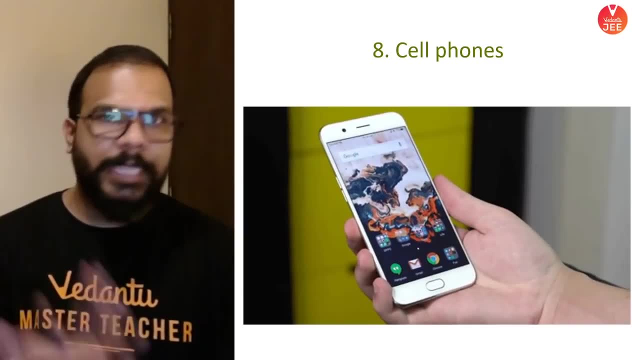 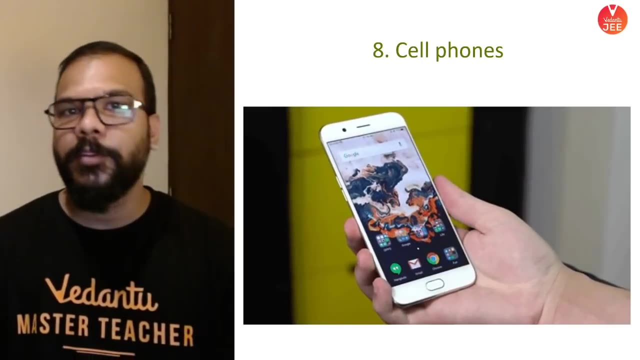 connected through different devices. There is a satellite which is also revolving around earth, which is also making this communication possible. So, if you want to look at it as a gadget, yes, it is working on the principles of electronics and semiconductor devices that we study in 12th. 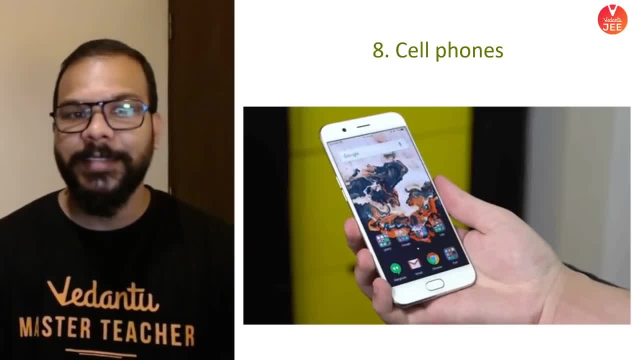 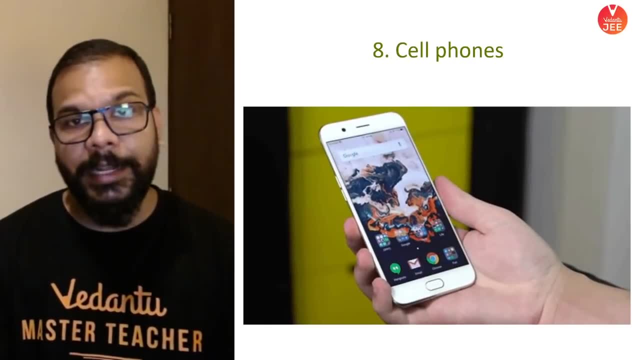 standard. In fact that is the last chapter of your physics in 11th and 12th standard. But if you look at it as a communication device, then that communication is possible because of the electromagnetic waves, precisely radio waves, which from your cell phone goes to the nearby. 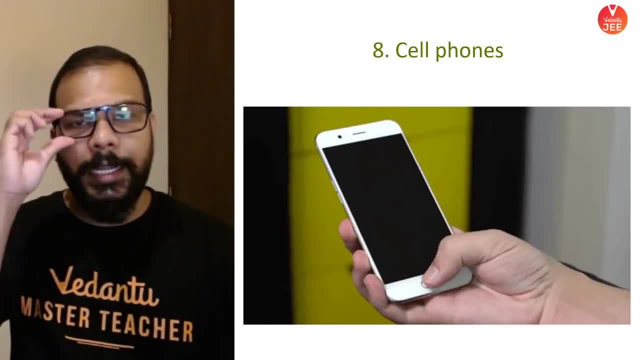 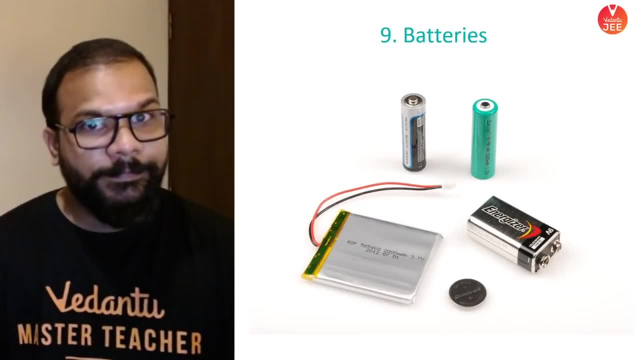 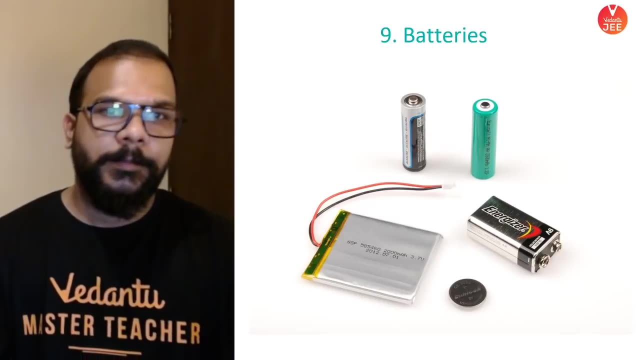 tower of your service provider. from that tower it goes to the satellite and from satellite it goes to that person whom you are trying to connect to. Moving on, yes, the energy storing devices: batteries. You know that batteries are very, very, very essential part of all the. 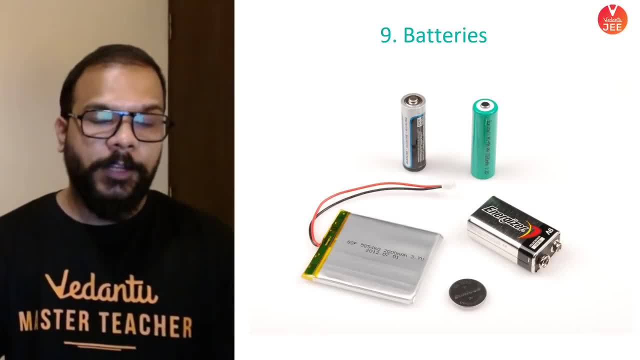 electronic and electrical devices that we use. In fact, one of the most preliminary and fundamental laws that we learn earlier in our school studies is what is the basic principle of working of any battery, and that is law of conservation of energy. So whenever you are trying to store the energy, 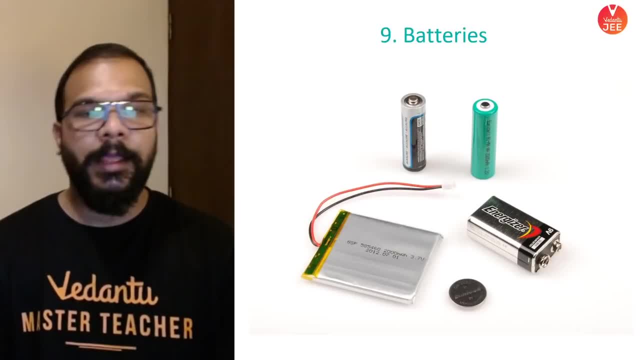 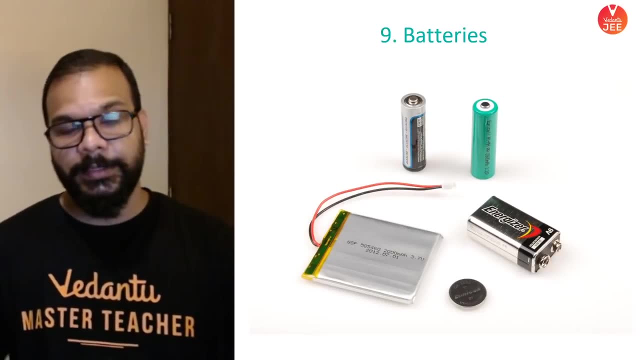 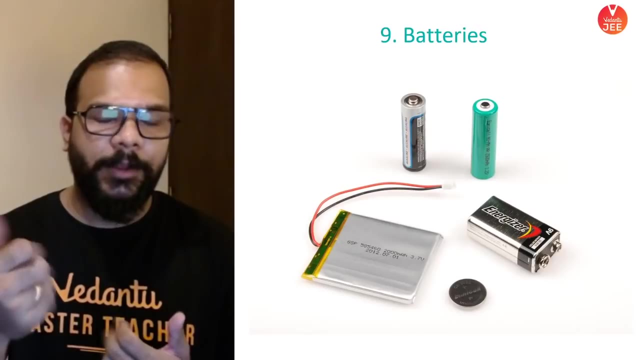 here you are storing the energy in the form of chemical, or you can say the potential energies of the chemical or ions, and then when you connect a battery to a circuit, that energy is being transferred to different devices. If this battery is going to get connected to a hand ceiling fan. 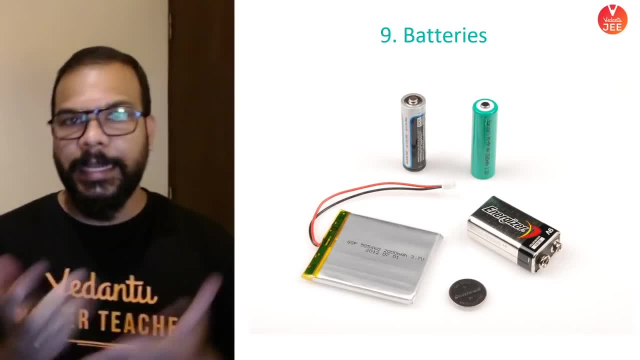 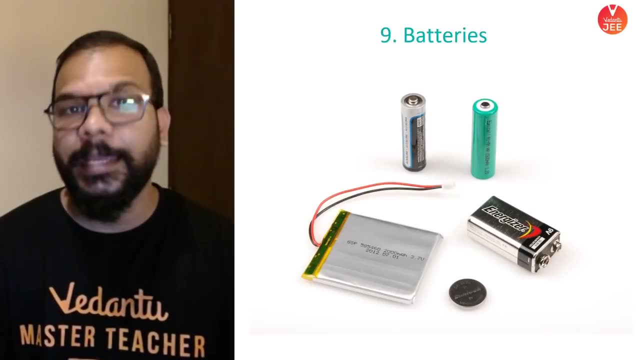 or not ceiling fan but hand fan, then that fan will create that chemical energy into electrical energy and that electrical energy will be finally converted into the mechanical energy of the fan. If you are going to connect it to a remote control, it is going to again convert it into the electrical 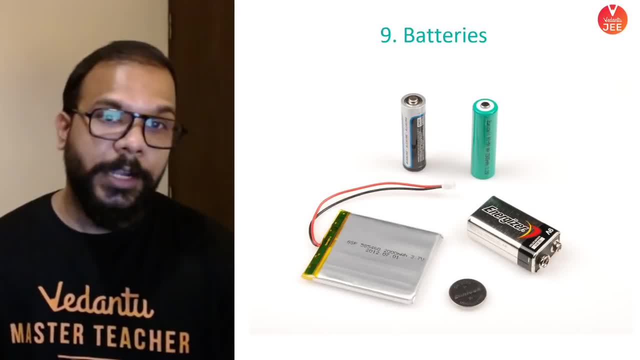 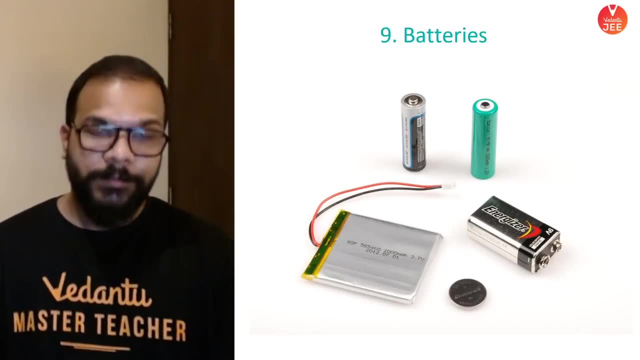 energy, which will eventually send the signal in the form of electromagnetic waves, so that your devices will be connected remotely. You know how important the batteries are. Remember they are working on the principles of law of conservation of energy And, last but not the least, is this: 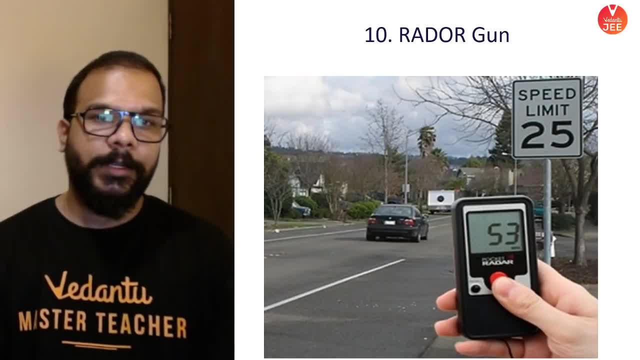 example that I have picked. It is a radar gun, or a gun which is used to measure the speed of any object. Now, this is a very interesting concept or phenomena, which we call as Doppler's effect. If you have not studied it in 11th standard so far, then you might not. 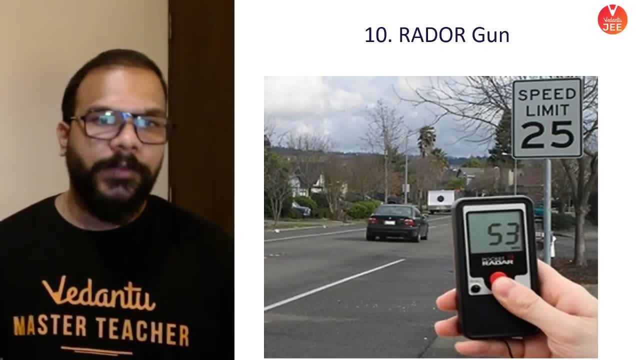 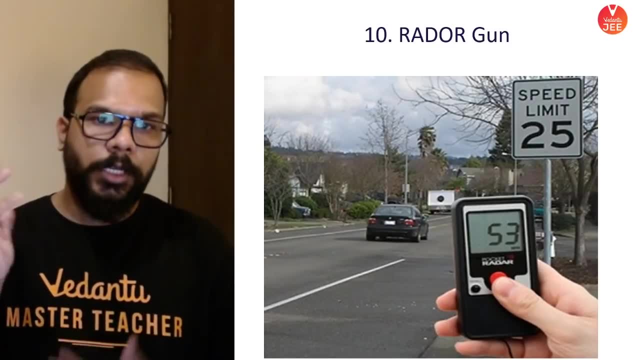 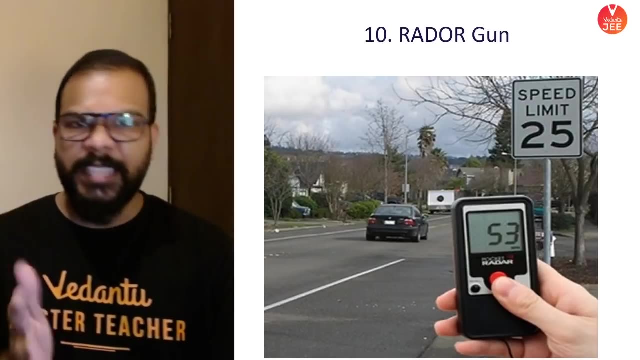 have even heard about it. Doppler's effect works on the variation of the frequency whenever there is a relative motion between the source which is producing the sound and the object which is receiving that sound. So in this case you send a sound signal. it hits the object with a certain 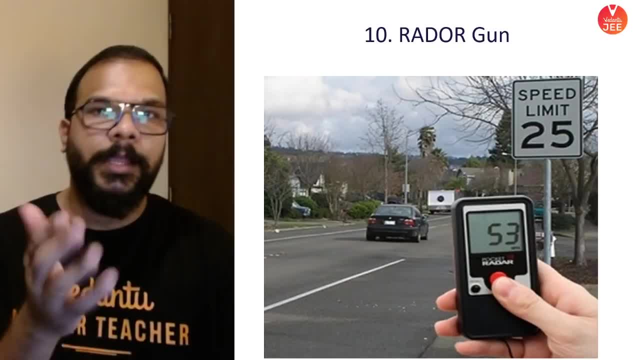 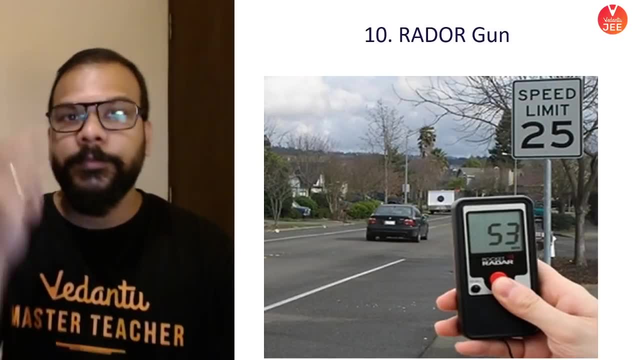 frequency you are generating that sound, it hits the object. If it comes back with the same frequency, that simply means that the object is not moving. But if there is a relative motion, then you will be able to calculate the speed with which the object is moving. 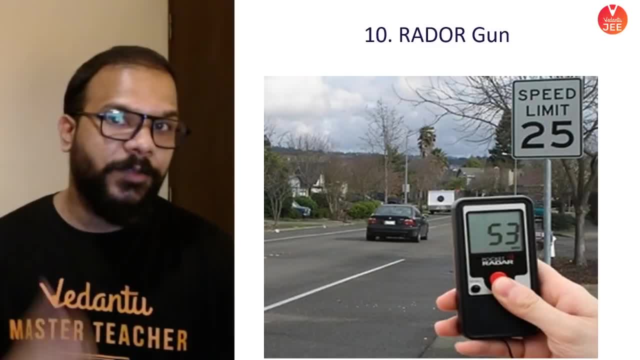 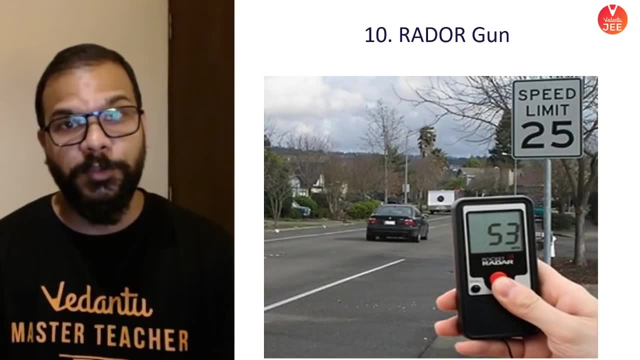 with the help of the difference of the frequencies which was sent and which was received. Yes, that's the beauty of something that we call as Doppler's effect, and with that you are able to calculate the speed with which your object was moving, So you can check whether there was over. 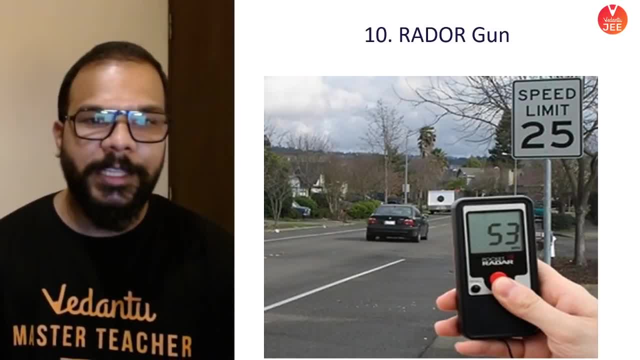 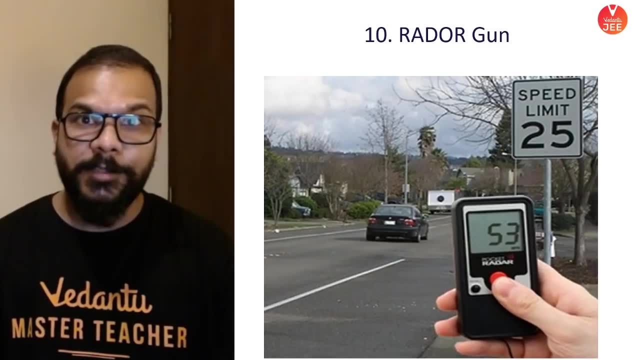 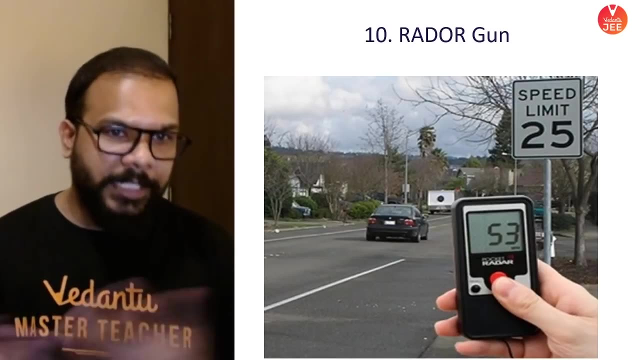 speeding or not. So that's why it's a useful device for the traffic police as well. In fact, it's not just used by traffic police. it is also used in cricket matches to measure how much the speed with which a bowler is bowling a ball- Cool people. So these were the 10 examples that 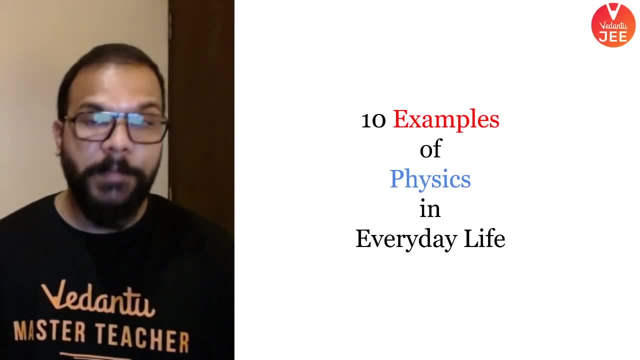 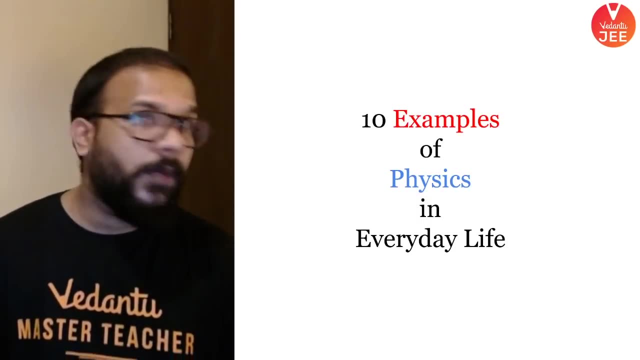 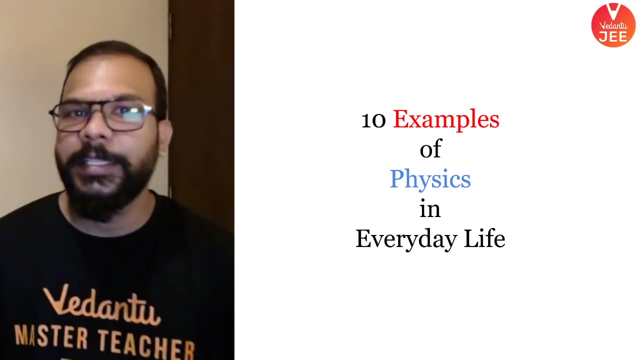 I could think of. I'm sure there would be many more that you are aware about. So if you, after watching this video, are thinking about certain things, if you are watching things around you and you are able to observe and figure out the law which is working behind those things, that 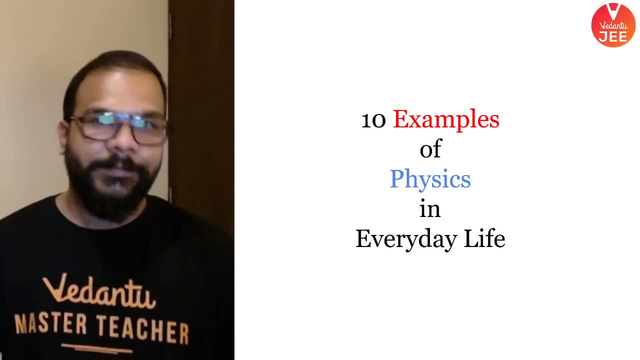 you are observing. do tell me that in the comment section, with the example and with the law or the concept of physics which is making that possible. So I would definitely and very eagerly be waiting for your comments in the comment section of this video. 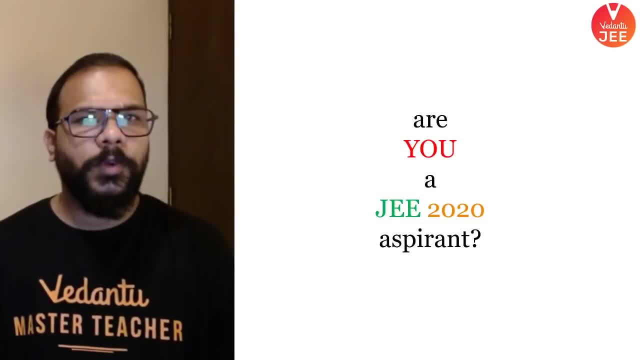 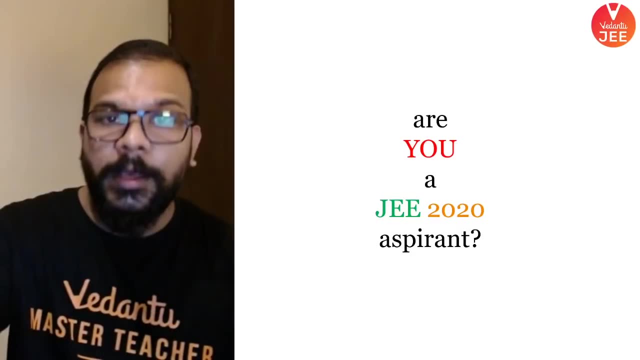 Now, before I say goodbye, I want to ask you: are you a J-2020 aspirant? Among you people? definitely there will be J-2020 aspirants who are watching this video. So, guys, you, I know. 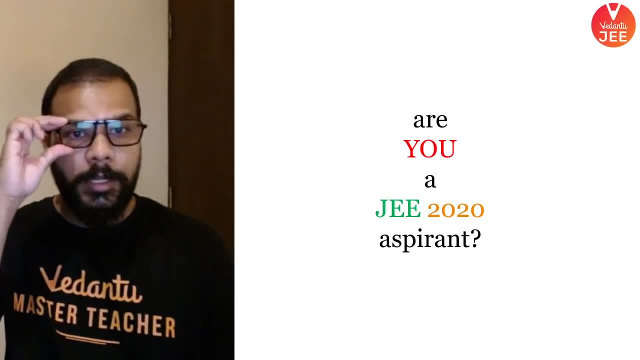 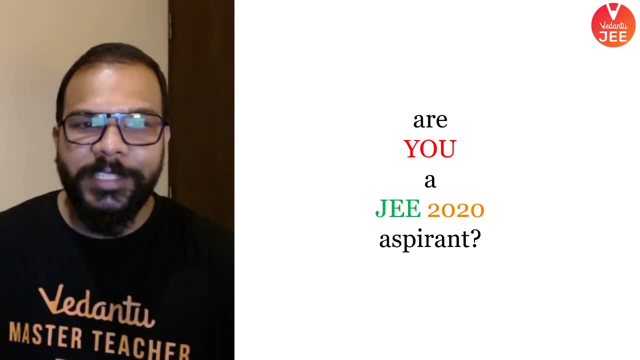 you guys are going through a crucial time. Your examination has already got postponed twice. Now it is being scheduled to happen in the month of September and some of you must be looking for a last-minute preparation. So for the final lap of preparation, guys, you can come to Vedantu's. 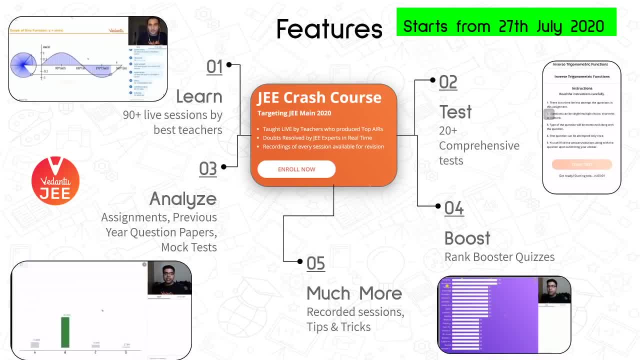 platform and that is our crash course. So, if you are interested in joining Vedantu's crash course- you have been wondering about it but haven't joined it yet. So, as a good news, coming Monday- yep, tomorrow itself- we are starting a fresh batch of crash course where you will be getting 90 plus. 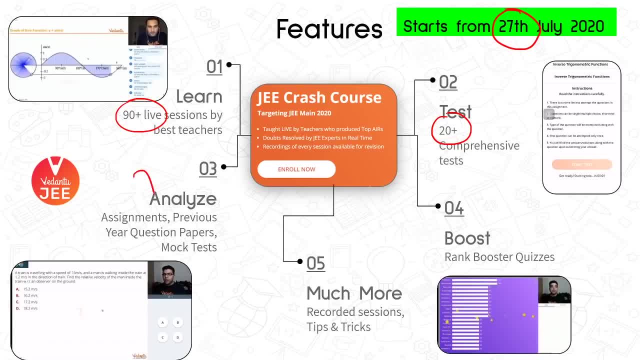 sessions: 20 plus tests as a test series. You will get the performance analysis of your own. You will have rank booster quizzes and much more, including recorded sessions, the replays of any sessions which happen over here. So if you missed out on the crash course earlier and you want to, 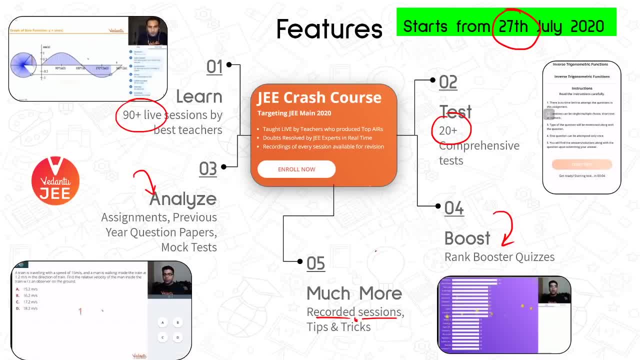 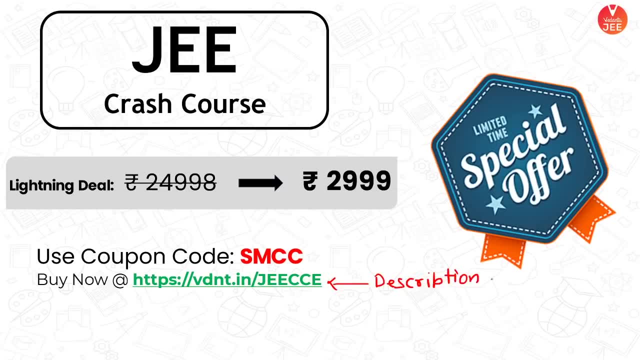 join. now it's possible again. What you are supposed to do for that? all you have to do is go on this link, which is available again in the description box along with that registration page: masterclass. This is also available in the description box. Click on that, It will take. 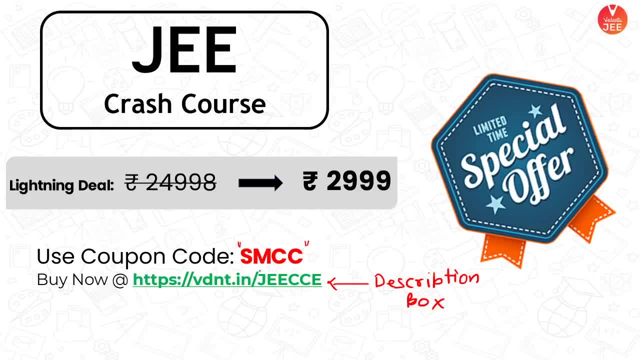 you to a new page where you will have to put this coupon code- don't forget it- SMCC. So the crash course, whose actual worth is almost 25,000, would not be that anymore and you will get the crash course for just under 3000 rupees. Okay, people. So I hope it will help you out and you will take